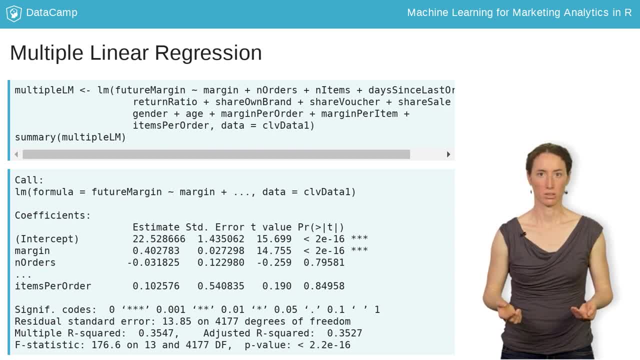 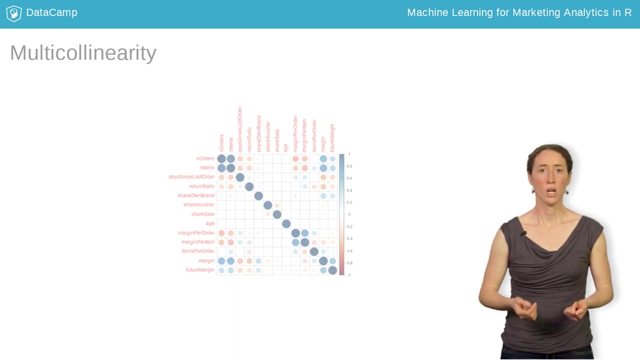 and so on. We save the model as multiple-LM. Just as before, we use summary now with multiple-LM as an argument. That worked, Although we now encounter other problems. Multicollinearity is one threat to a multiple linear regression. This occurs when the model is modeled as a function of. 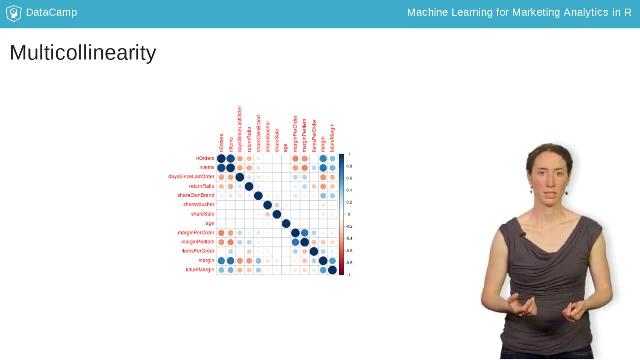 This occurs whenever one explanatory variable can be explained by the remaining explanatory variables. Then the regression coefficients become unstable and the standard errors reported by the linear model are underestimates Due to high correlation between n orders and n items, as well as margin per order and margin per item. 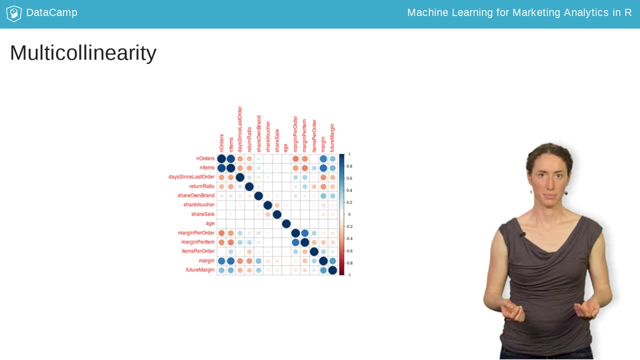 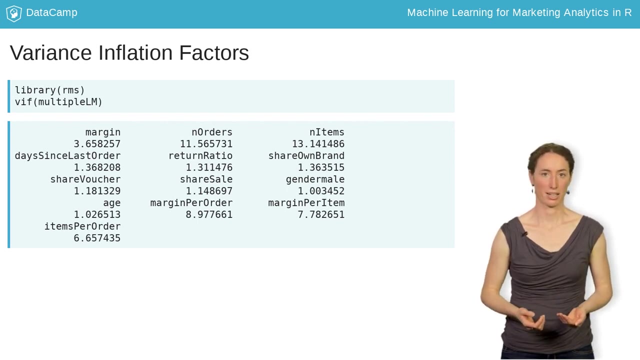 these variables are candidates for multicollinearity. To systematically check all variables in a model for multicollinearity, we calculate the variance inflation factors using the with function from the RMS package. These indicate the increase in the variance of an estimated coefficient due to multicollinearity. 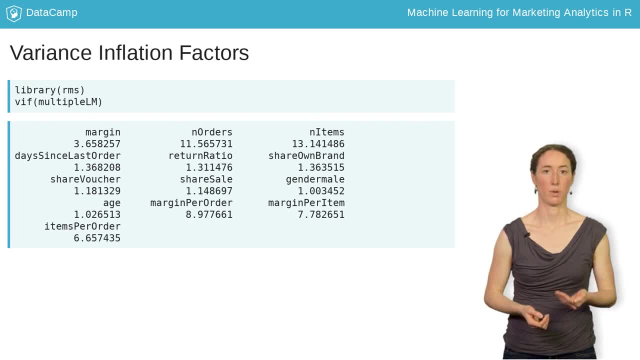 A with higher than 5 is problematic, And values above 10 indicate poor regression estimates. Let's look at our model's variance inflation factors. As expected, the widths for n orders and n items, as well as margin per order and margin per item, are rather high. 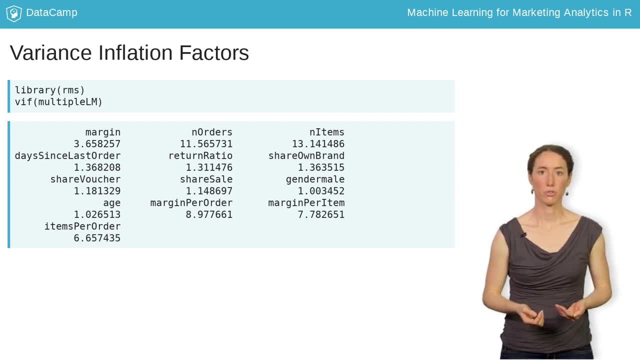 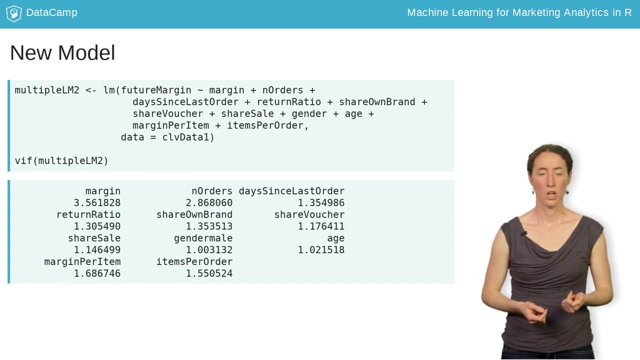 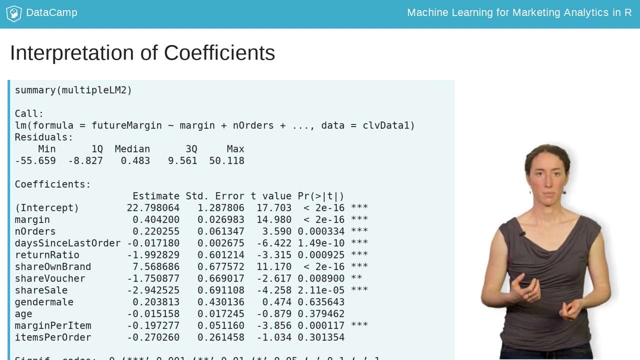 Hence we exclude one of each pair from the regression, namely n items and margin. per order. Here are the widths of the new model. They are all acceptable. now, Finally, we are ready to interpret the model output. The intercept gives the expected margin in year 2 when all independent variables are set to 0..